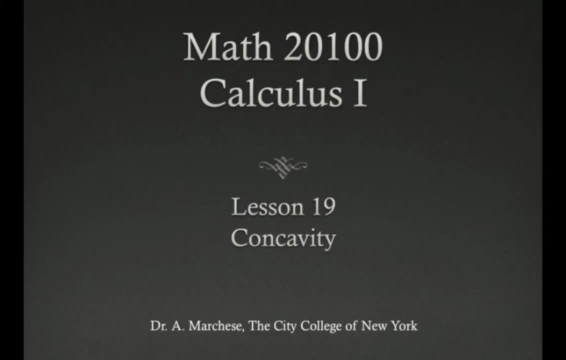 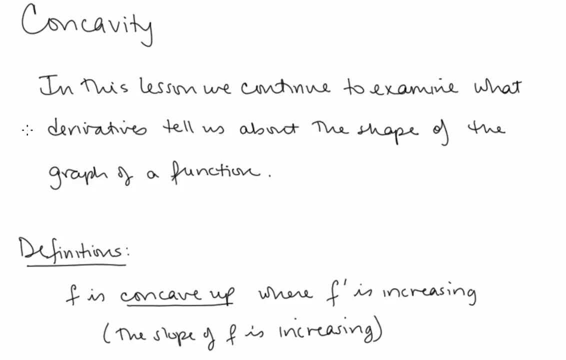 This is lesson 19 in our Calculus 1 series: Concavity. In this lesson we continue to examine what derivatives tell us about the shape of the graph of a function. Let's take a look at this definition. F is concave up where F. 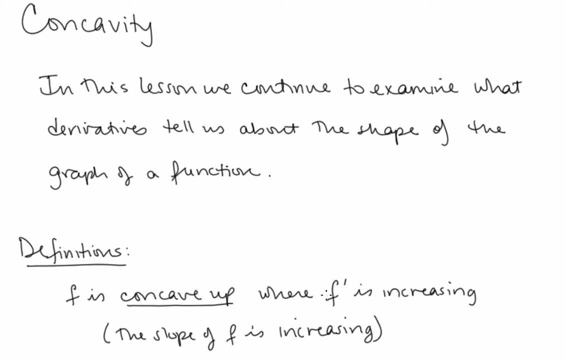 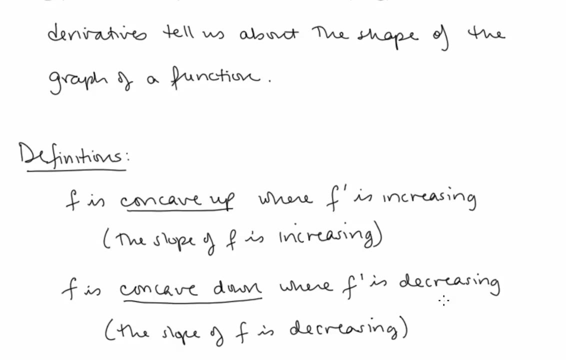 prime is increasing. Remember that F prime gives us the slope of F. so what we're saying here is that the slope of F is increasing. That's what we call concave up. Similarly, concave down is where F prime is decreasing. so where the slope of F is decreasing, Let's 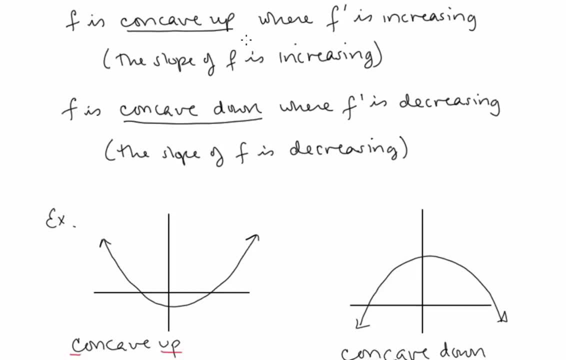 take a look at the pictures here. Concave up has the slope increasing, So we can see here that the slope starts at a steep negative slope and then becomes less and less negative and then turns that slope into a steep negative slope, so that trade-off is towering and 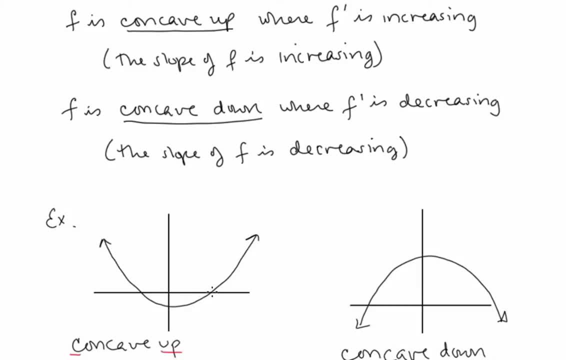 is estate in this Fundstein equation, just like the vớiy어논의oid equation, to 0 slope, more and more positive. So the slope here is increasing. Here we have a high positive slope which is decreasing to 0 slope. 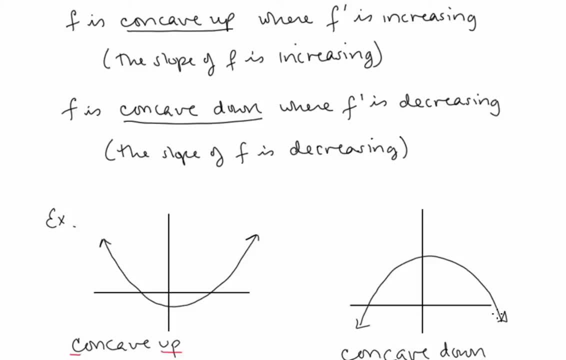 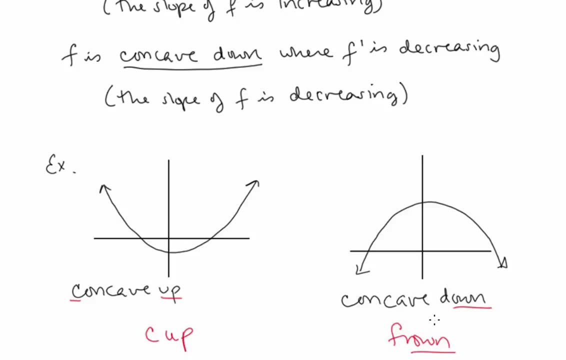 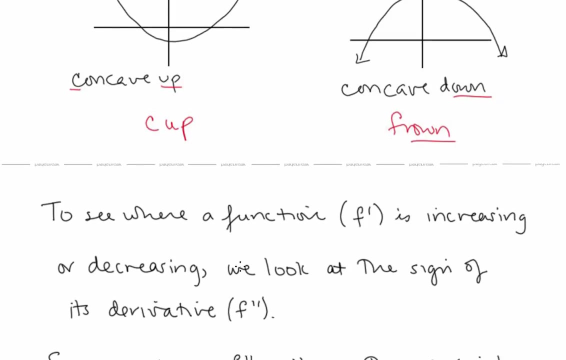 and then to a negative slope. And an easy way to remember which is which concave up is cup-shaped and concave down is shaped like a frown. Now to see where a function is increasing or decreasing, we take a look at the sine. 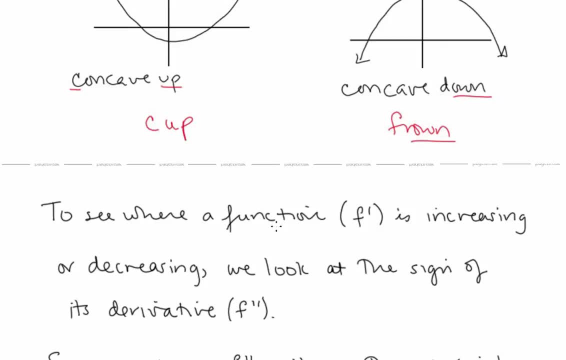 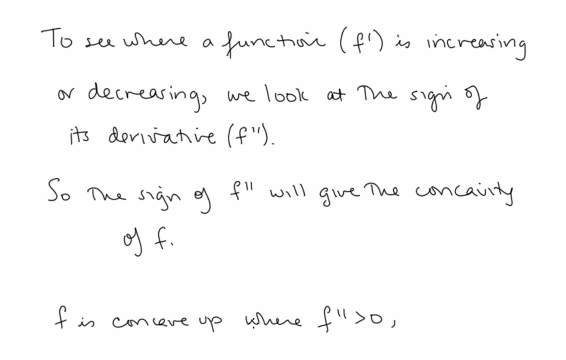 of its derivative. So to see where f prime is increasing or decreasing, we want to look at the sine of its derivative, f double prime. So the sine of f double prime is going to give us the concavity of f. F is concave up. 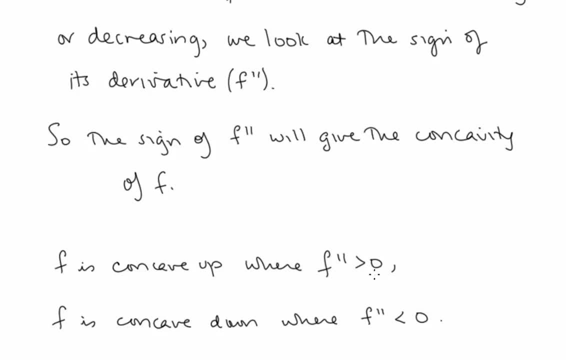 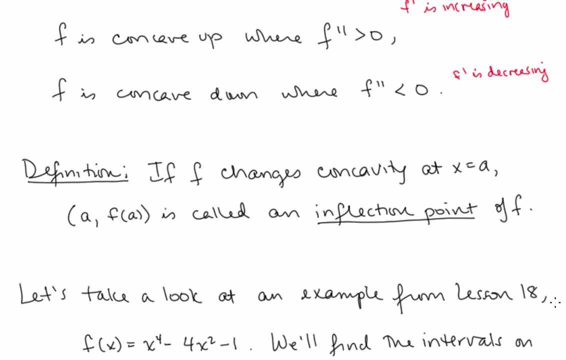 where f double prime is positive, This says that f prime is increasing And f is concave down. where f double prime is negative, This says that f prime is decreasing, And the point at which concavity changes is called an inflection point. 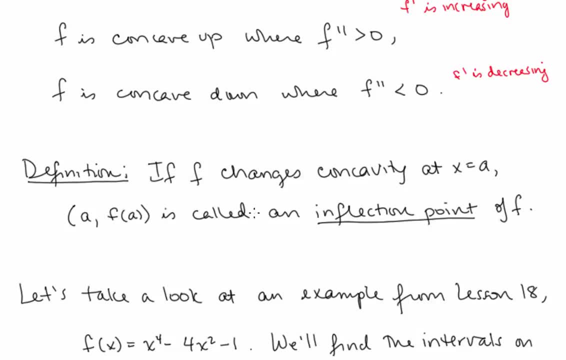 If f changes concavity at x equals a, then the point a comma f of a is called an inflection point of f. So let's take a look at an example we had in the last lesson: f of x equals x to the fourth minus 4x squared. 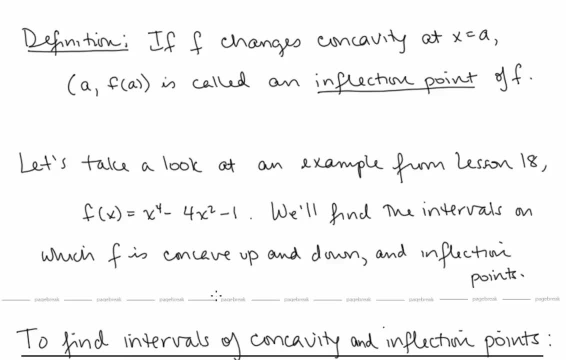 minus 1.. In the last lesson we took a look at intervals of increase and decrease and relative extrema. Now let's take a look at intervals on which the graph is concave up and concave down and find any inflection points. 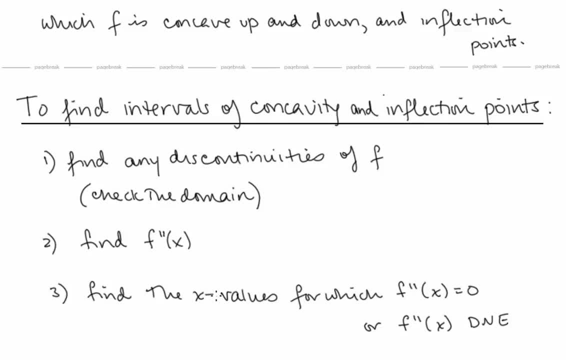 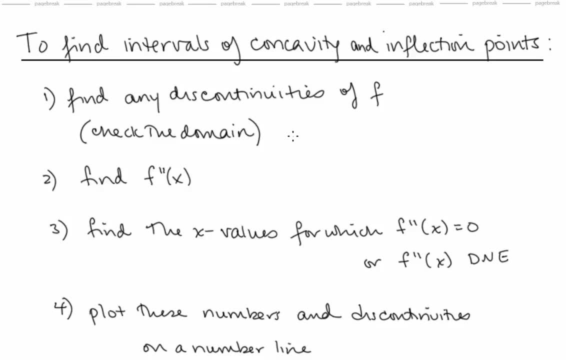 So to find intervals of concavity and inflection points. we want to find any discontinuities of f. So we'll check the domain Again. we're on the lookout for asymptotes. We want to find f double prime of x, Find the. 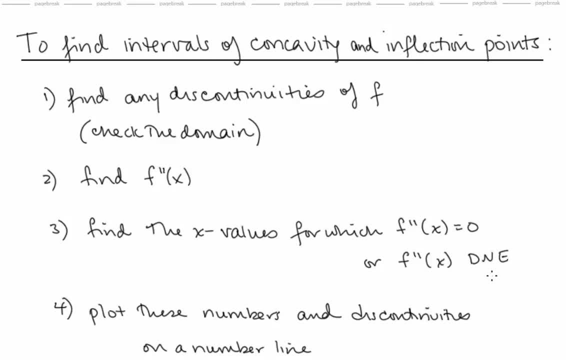 x values for which the second derivative is equal to zero or does not exist. Remember, for the first derivative, these were called critical numbers. We don't have a name for them. for the second derivative, We want to plot these numbers and any discontinuities on a number line. 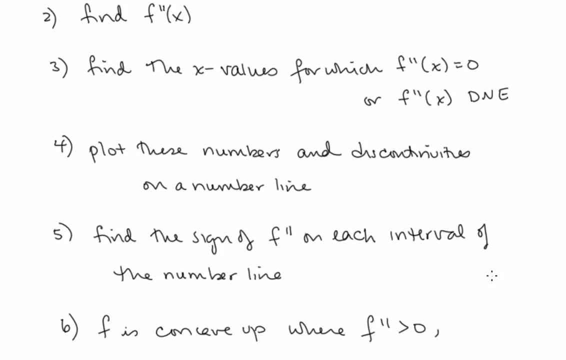 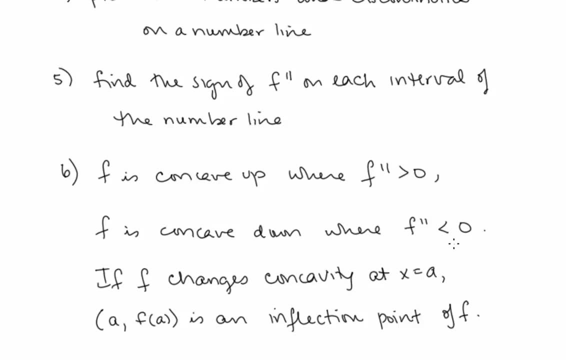 and then check the sign of f double prime on each interval. f is concave up where f double prime is positive. f is concave down where f double prime is negative, And if f changes, concavity at x equals a. f of a is an inflection point of f. So keep in mind, here we're. 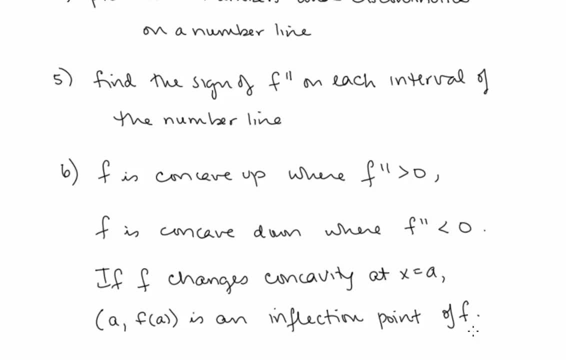 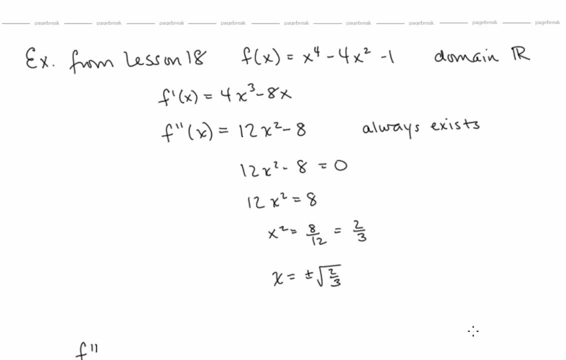 only calling a point, an inflection point, if there is a change of concavity. So let's take a look at this example. We found our first derivative to be 4x to the third minus 8x, And so our second derivative is 12x square. 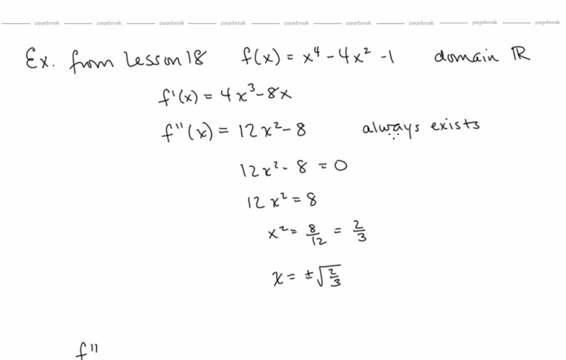 minus 8. And so we notice that this always exists, And so we set it equal to zero. to find any possible solution Solving for x. we have: x is equal to positive or negative radical two-thirds, So we set up a number line. 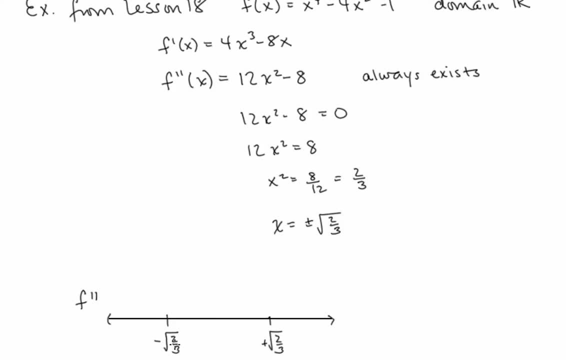 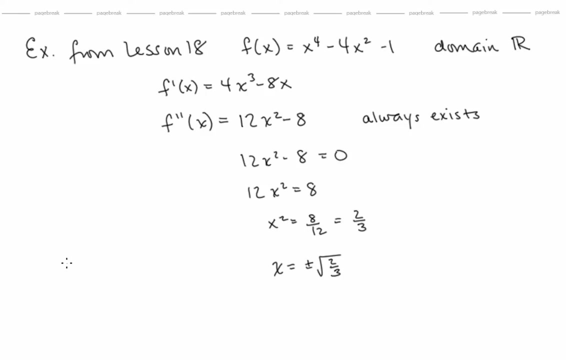 with our positive and negative radical two-thirds on the number line And we want to test the sign of f double prime. So on this interval let's choose. say x equals negative 1. f double prime of x is equal to 12x square. 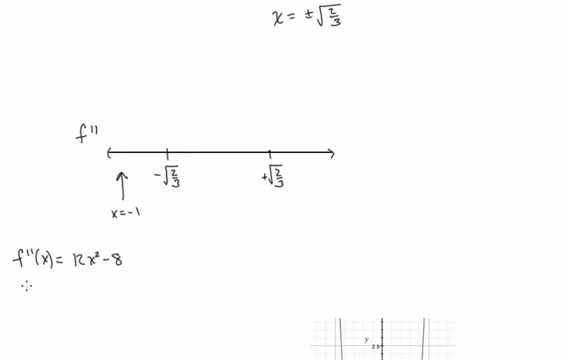 minus 8.. And so f double prime of negative 1 is equal to 12 times negative 1 square minus 8.. And that's going to be a positive number. So we'll put a positive sign here. Here let's choose: x equals 0.. f double prime of 0. 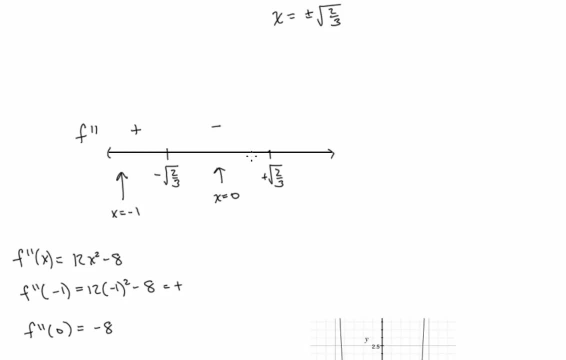 is going to be negative 8.. So that's negative, And here let's choose: x equals 1.. We have the same computation here as for negative 1.. f, double prime of 1 is going to be 12 times 1 square. 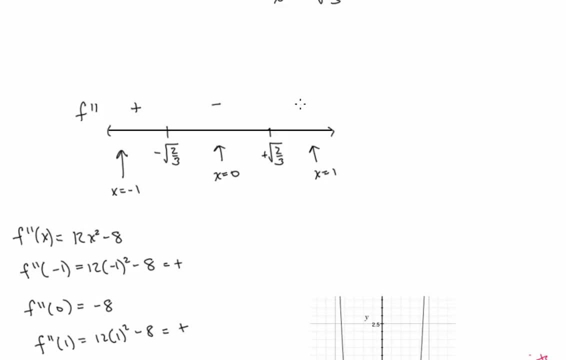 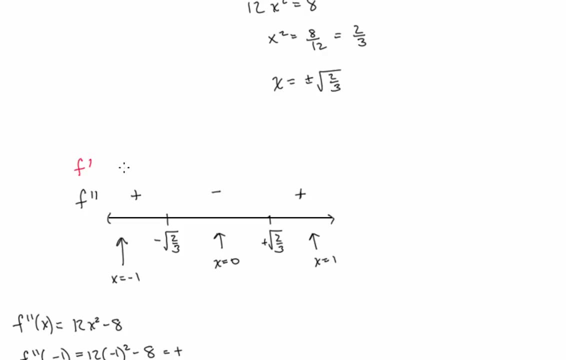 minus 8,, which is 4,, which is positive, And so we put a positive sign here. So this tells us that f prime is increasing, then decreasing, then increasing, And so that tells us f is concave up, then concave down. 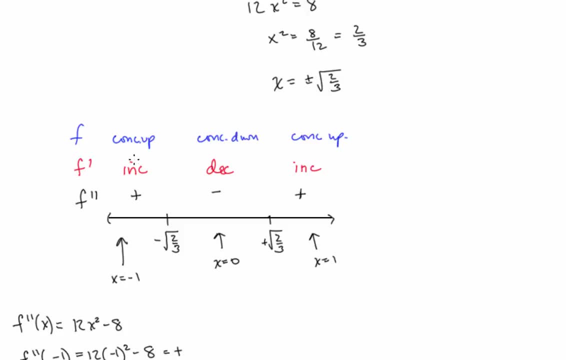 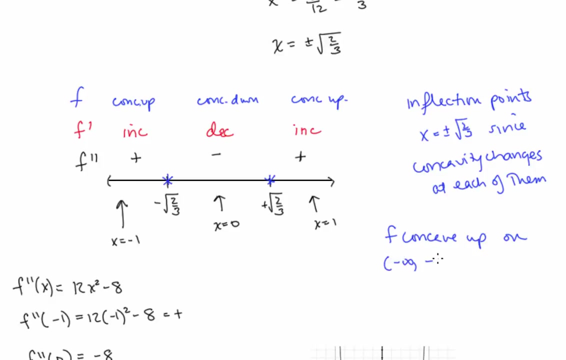 Now notice we have a change of concavity at both of these points. So they are both inflection points And we can say: f is concave up on negative infinity to negative radical two-thirds union, positive radical two-thirds to infinity, And f is concave down on negative radical two-thirds. 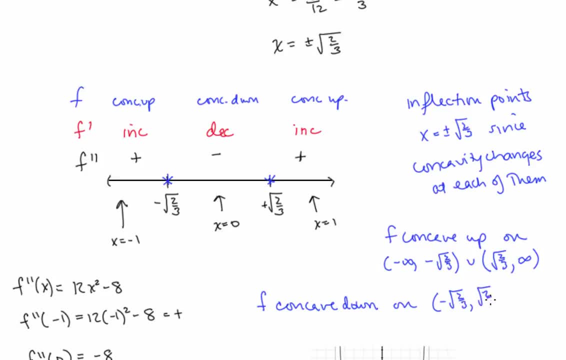 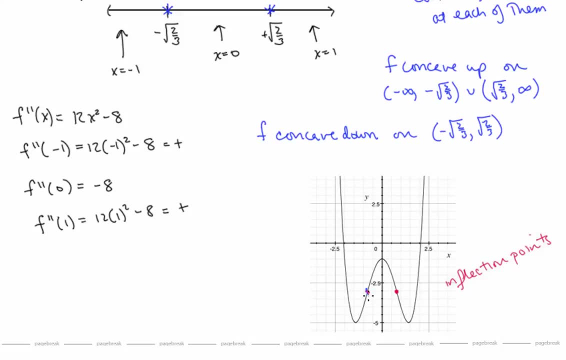 And remember that our graph looks like this, And so here are our inflection points: f is concave up on negative infinity to negative radical two-thirds, Then it's concave down to radical two-thirds And then it's concave up again. Let's take a look at another example. 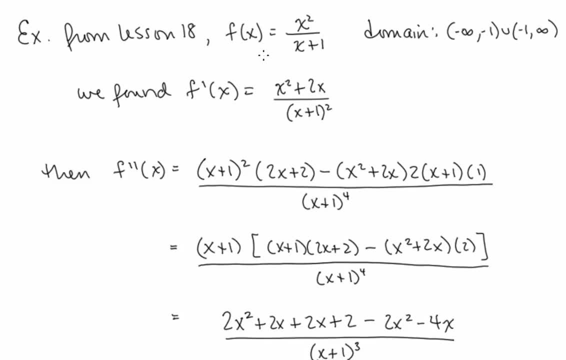 This one is also from lesson 18.. f of x is equal to x squared over x plus one. We found in the last lesson that the domain here is negative infinity to negative one, union negative one to infinity, and that we have an asymptote at x equals negative one. 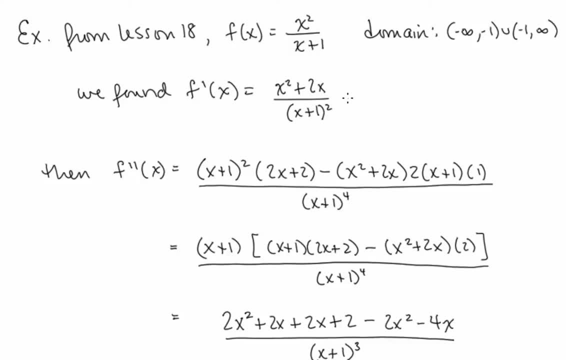 We found the first derivative to be x squared plus two, x over x, plus one quantity squared. And so now for concavity. we want to find the second derivative. So we're going to use the quotient rule here: Bottom times derivative of the top minus top times derivative of the bottom over bottom squared. 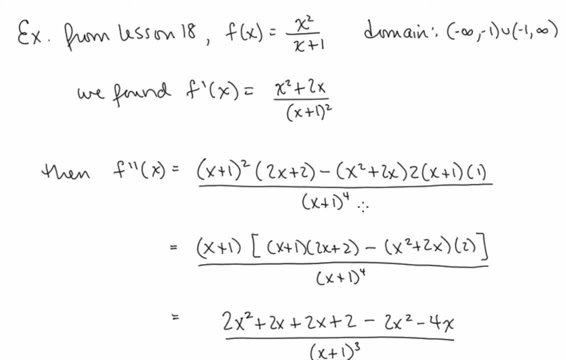 Remember that we're going to be seeing where this does not exist and also where it is equal to zero. So we're definitely going to want to set the numerator equal to zero, and factoring usually helps us solve. But here we also notice that we have a factor of x plus one in both terms in the numerator. 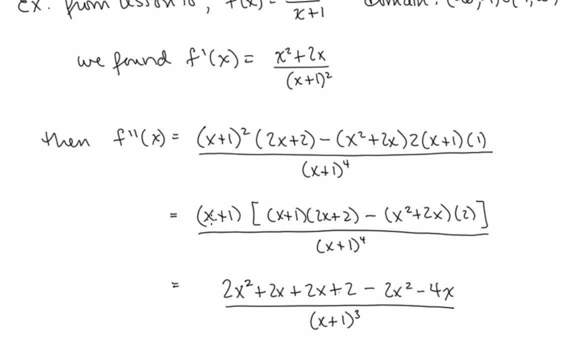 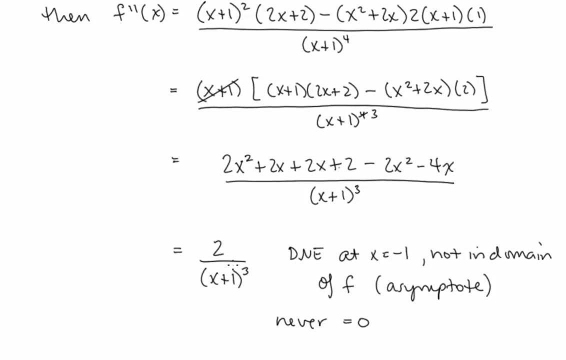 that can cancel with one in the denominator. So now we're here, and since the powers are all quite low, it's easiest to multiply out and simplify that way. So we multiply out here As well as here, and we simplify and we're left with just a two in the numerator. So we have two over x plus one to the third. 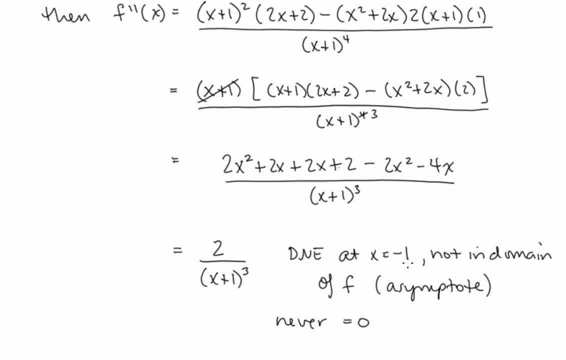 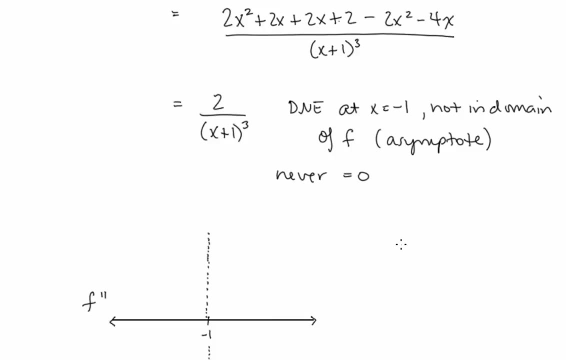 and we realize this does not exist. at x equals negative one, and that's an asymptote. We found that already, And this can never equal zero. So the only number that needs to go on our number line is the asymptote. at x equals negative one. So we're here. 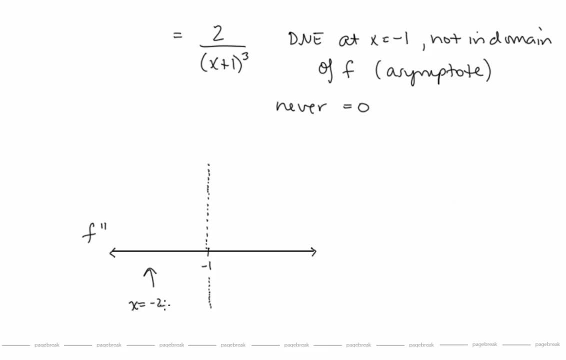 And so here let's take: x equals negative two, F double prime of negative two is going to be two over negative two, plus one quantity to the third, That's two over negative one to the third, and that's going to be negative. Here let's take, say x equals zero. 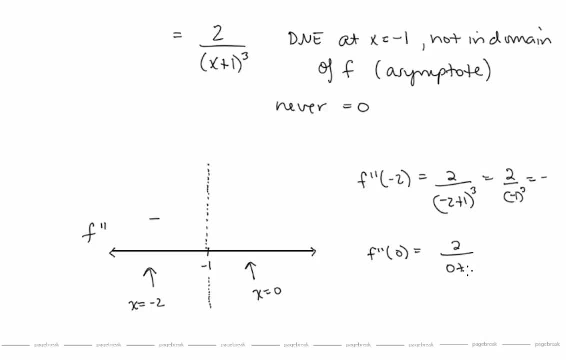 F double prime of zero is two over zero plus one to the third and that is going to be positive. So this tells us that f prime Is decreasing and then increasing And that f is concave down before the asymptote and concave up after the asymptote. 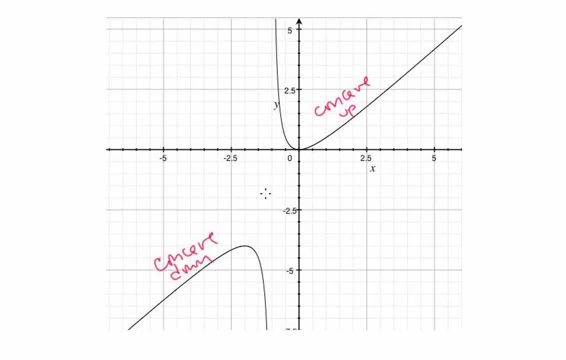 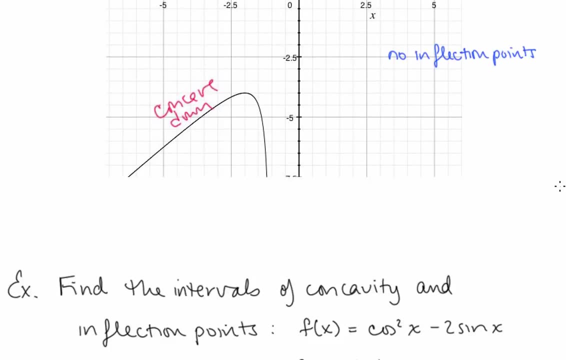 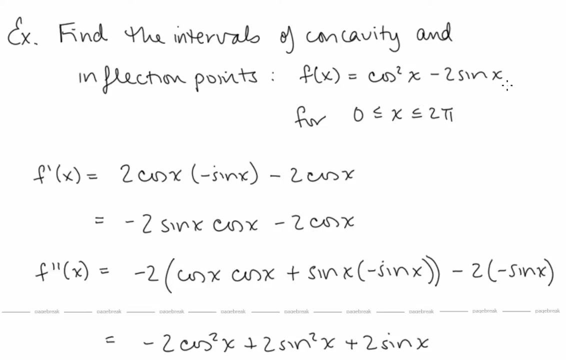 And if you recall, our graph looks like this: Here we have no inflection points. Let's take a look at another. Find the intervals of concavity and inflection points. for f of x equals cosine square x minus two, Two sine x over the interval x between zero and two pi. 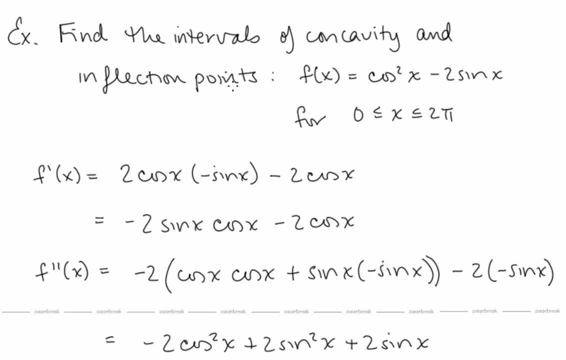 So if we're looking for concavity and inflection points, you want the second derivative, So we'll start by taking the first derivative. So the two comes down. We have two cosine x times negative sine x, Minus a two cosine x. 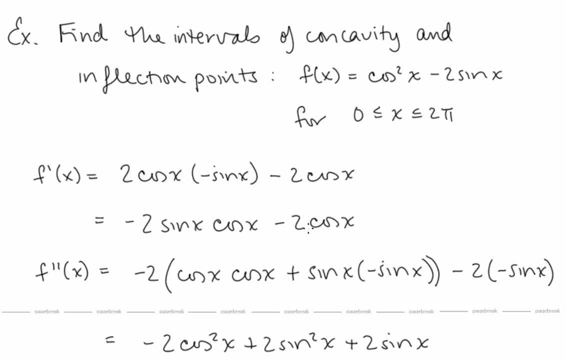 So we have negative two sine x, cosine x, minus two cosine x, And you could either factor from here and then continue, Or you can simply just take the derivative from here. I took the derivative straight from here And notice, I left my negative two on the outside and I used the product rule on the inside. 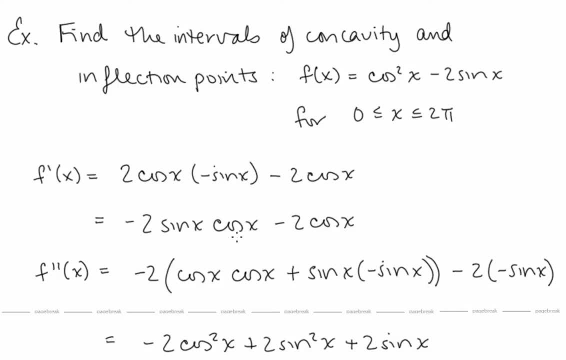 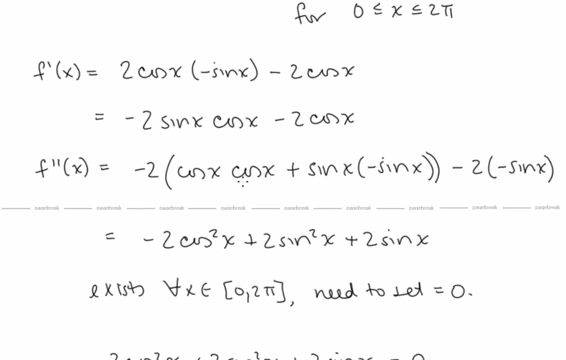 of those parentheses. So I was using the product rule just on sine x, cosine x. So I had derivative of the first times the second plus first times derivative of the second. Then here we have a negative two times a negative sine x. So multiplying through the negative two we have negative two cosine square x. 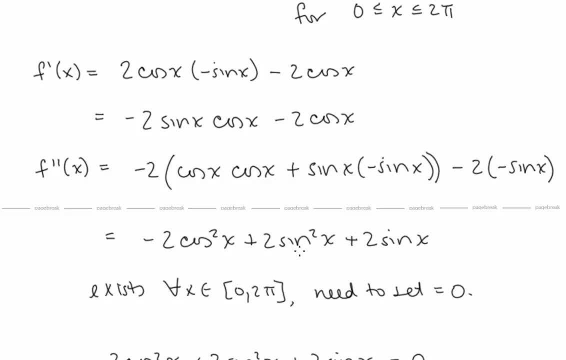 Then we have negative two times negative, that's a positive: two sine square x plus two sine x, And the first thing we notice is that this exists for all x in the given interval zero to two pi, And so we need to set this equal to zero. 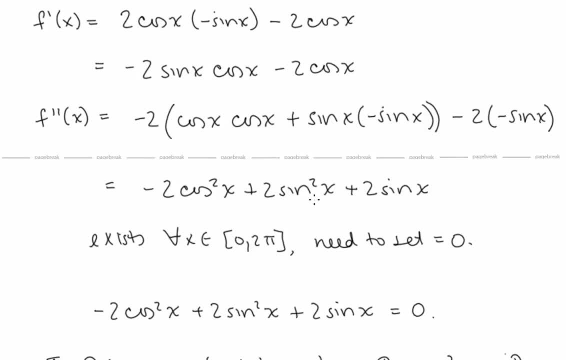 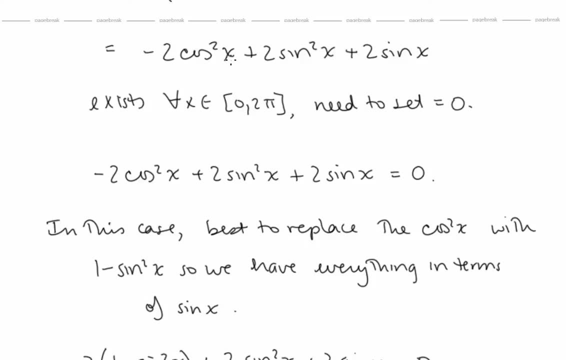 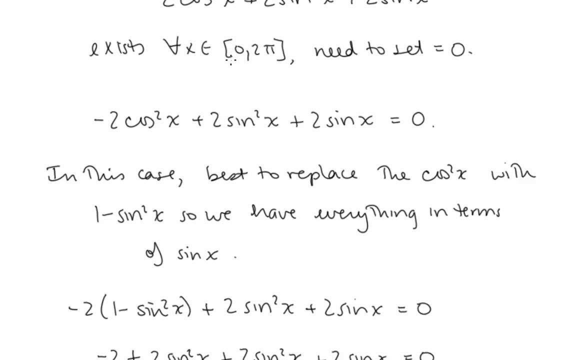 Now how are we going to solve this? equal to zero if we have both sines and cosines involved. The best way to do it is to Replace this cosine square x with a one minus sine square x, So everything will be in terms of sine x. 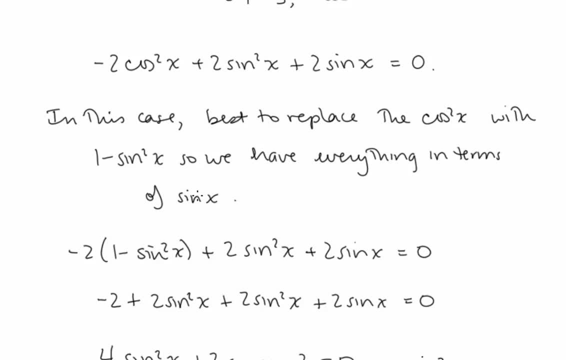 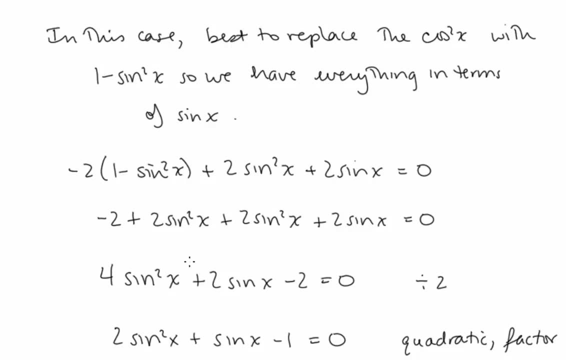 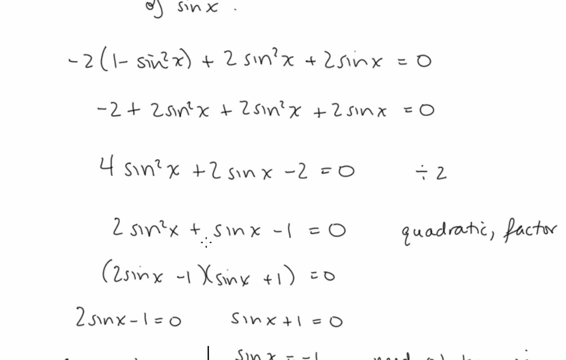 So replace the cosine square x with one minus sine square x. And so we're here. Distribute through the negative two, Combine like terms And we can divide by a factor of two here to simplify even further. And now we have a quadratic in sine x. 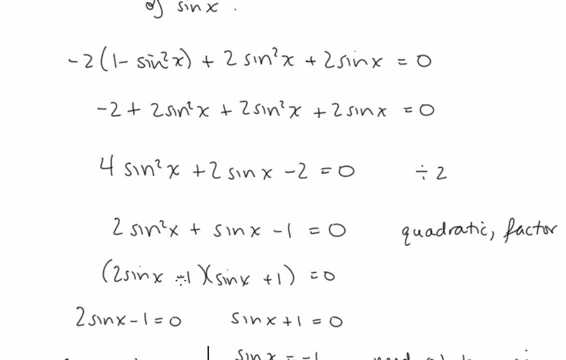 And so now we factor and we have 2 sine x minus 1 multiplied by sine x plus 1.. And that product is equal to 0.. So either 2 sine x minus 1 is equal to 0, or sine x plus 1 is equal to 0.. 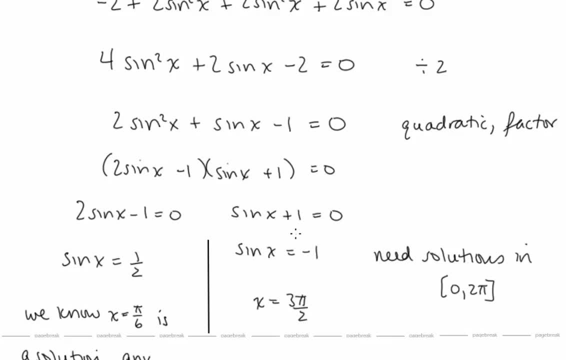 On this side we have: sine x is equal to negative 1. And we know that the only solution in 0,, 2 pi is when x is equal to 3 pi over 2.. Think about your sine graph here. Here we have: sine x equals 1 half. 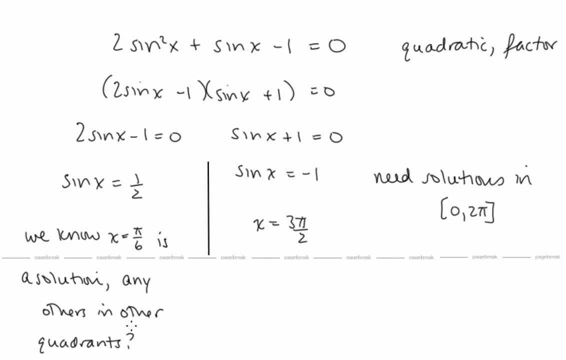 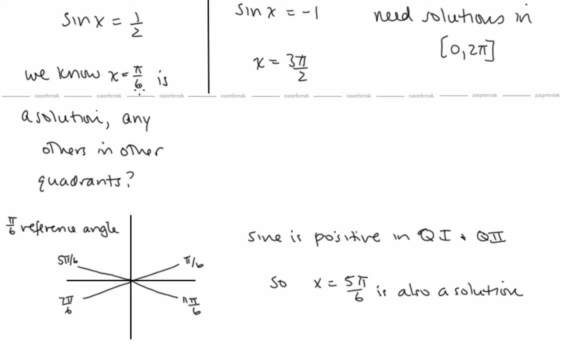 And we know that x equals pi over 6 is a solution. but we need to check the other quadrants because there is going to be another solution in one of the other quadrants. So how can we tell where the other solution is going to be? 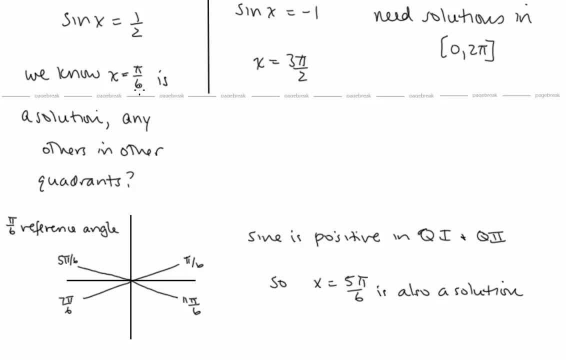 Well, we treat x equals pi over 6 as a reference angle. Draw that up in each quadrant. Here that's pi over 6.. Here that's 5, pi over 6.. Here it's 7 pi over 6.. 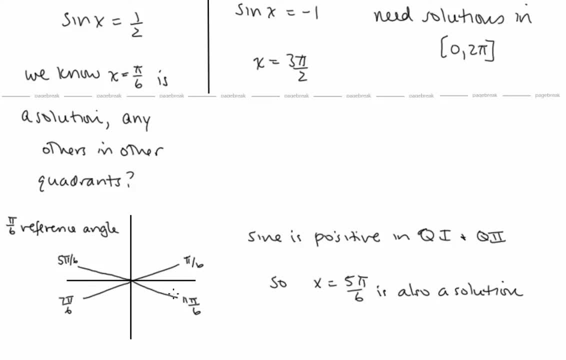 And here Here 11 pi over 6.. And now, which quadrants have sine a positive value? That happens in quadrants 1 and 2.. So the other solution is: x equals 5 pi over 6.. So we have three solutions here that are potential inflection points. 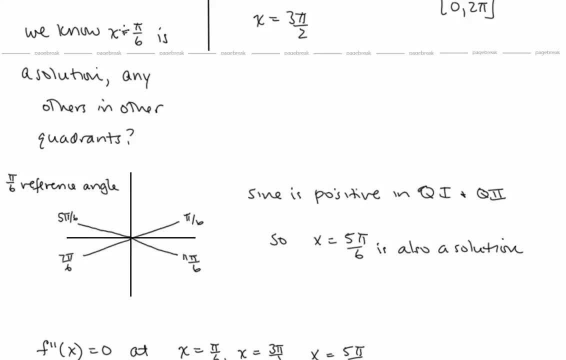 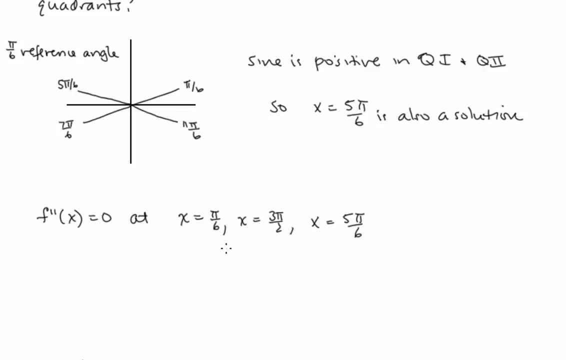 We still have to test them. on the number line. We have x equals pi over 6, x equals 5 pi over 6, and x equals 3 pi over 2.. These are the points. We have a point at which the second derivative is equal to 0.. 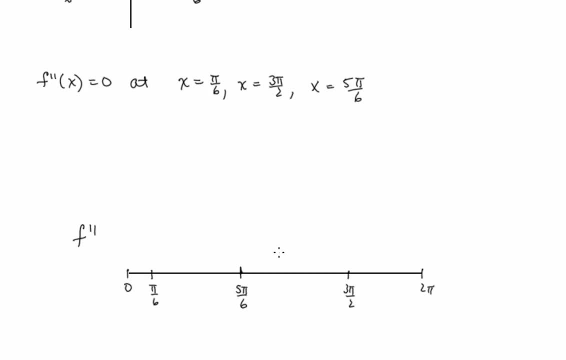 And so these go on our number line And notice we're on a restricted domain here from 0 to 2 pi. So I'm putting a 0 here and a 2 pi here instead of arrows on the number line. So now we need to test the sine of f double prime in each interval. 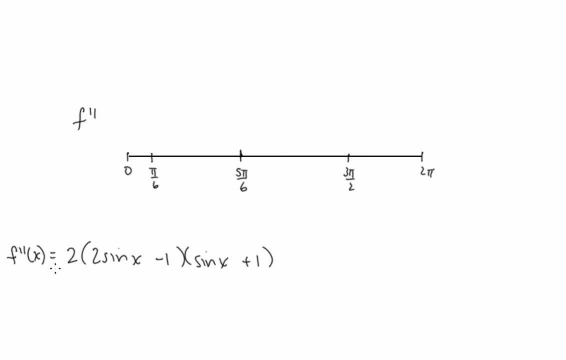 And to do that I'm going to use the factored form of f double prime. Now, to choose a point in the interval 0 to pi over 6, we can choose something like x equals pi over 8.. But notice, there's not going to be a convenient x value for which we know the sine values to make these computations. 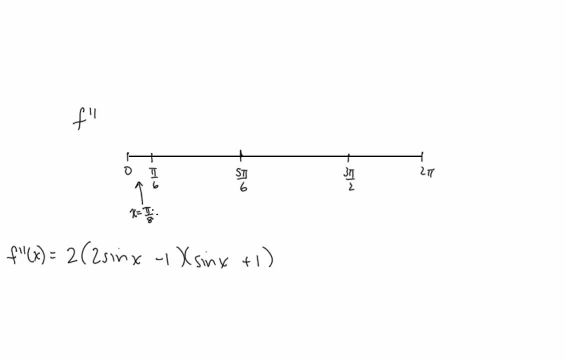 But that's okay. We can use our sine graph and figure out for x equals pi over 8 if these values are positive or negative. So let's take a look at our sine graph. We know that at pi over 6, sine of pi over 6 is 1 half. 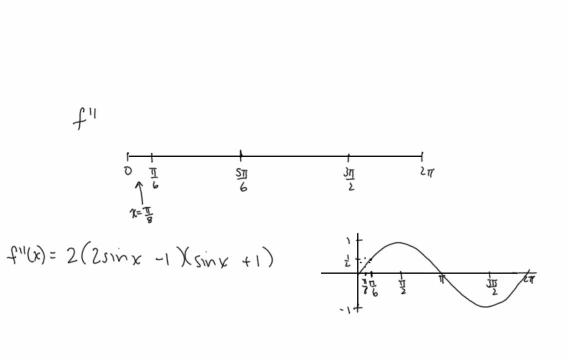 So at pi over 8, we know sine value is less than 1 half. So for f double prime of pi over 8, we have 2 times. We have this value less than 1 minus 1.. So this is going to be a negative. 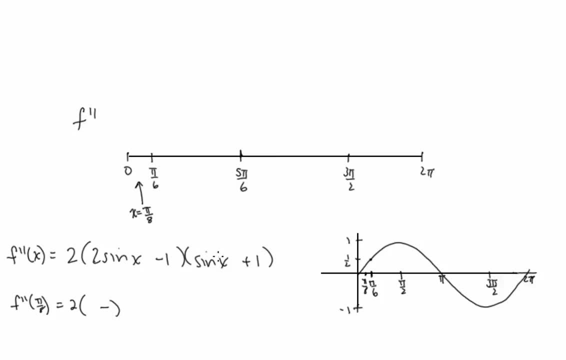 And then here we have a positive value plus 1.. So that's going to be positive, So this is going to be negative And f double prime is negative. on this interval Now between pi over 6 and 5 pi over 6, we could choose, for example, x equals pi over 2.. 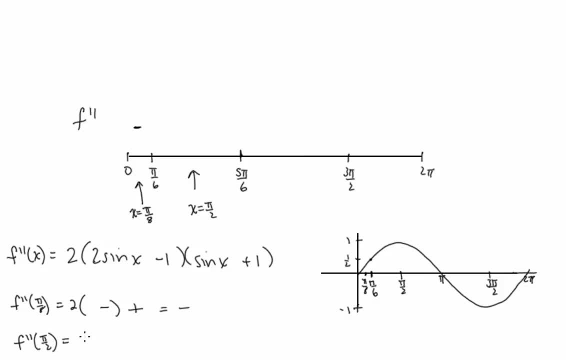 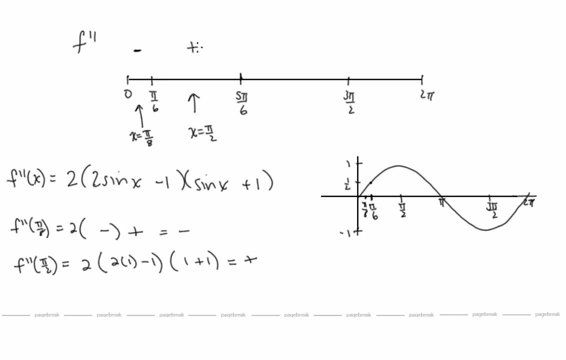 f, double prime of pi over 2 is going to be 2 times 2 times 1 minus 1, 1 plus 1.. So this is going to be 2 times a positive times a positive. That's all positive Between 5 pi over 6 and 3 pi over 2, we can choose: x equals pi. 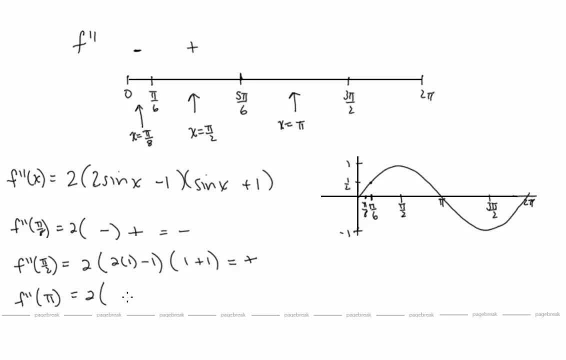 f, double prime of pi is going to be 2 times 0.. 0 minus 1 times 0 plus 1.. That's going to be negative And between 3 pi over 2 and 2 pi we can choose, say 11 pi over 6.. 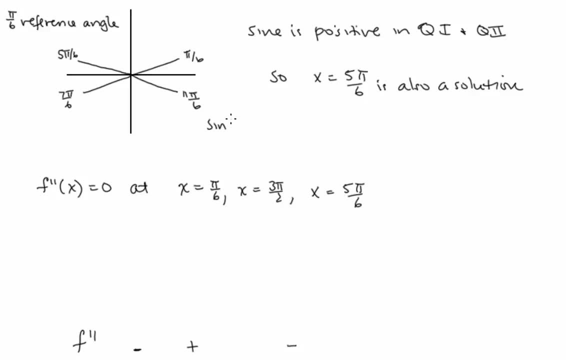 Right, That's this angle. And we know that sine of 11 pi over 6 is going to be negative of the sine of pi over 6.. So that's going to be negative 1 half. So f double prime of 11 pi over 6 is going to be negative of the sine of pi over 6.. 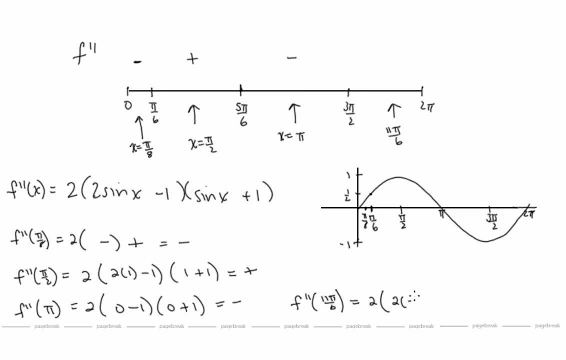 So that's going to be negative 1 half. So f double prime of 11 pi over 6 is going to be negative. So f double prime of 11 pi over 6 is going to be 2 times 2 times negative. 1 half minus 1 times negative. 1 half plus 1.. 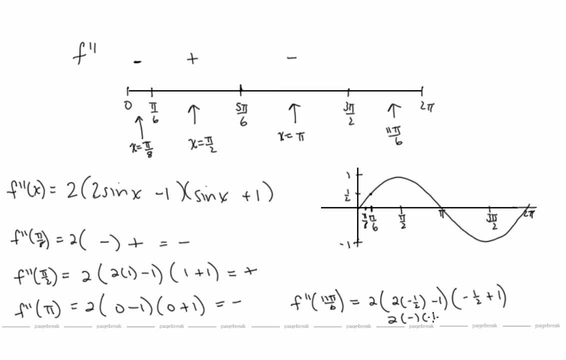 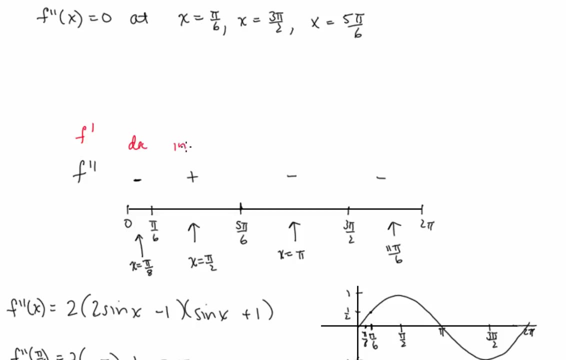 So this is going to be 2 times a negative, times a positive and that's going to be negative. Okay, so what does this say about f prime? This says that f prime is decreasing, increasing, decreasing, And it says that f is concave down, then concave up, then concave down and still concave down. 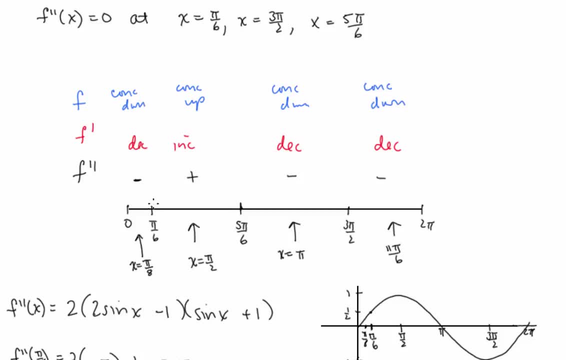 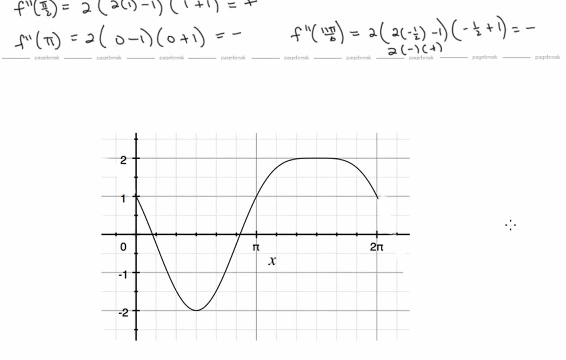 So we're going to have an inflection point at pi over 6.. We're going to have another inflection point at 5 pi over 6.. And no change in concavity at 3 pi over 2.. So let's take a look at the graph here. 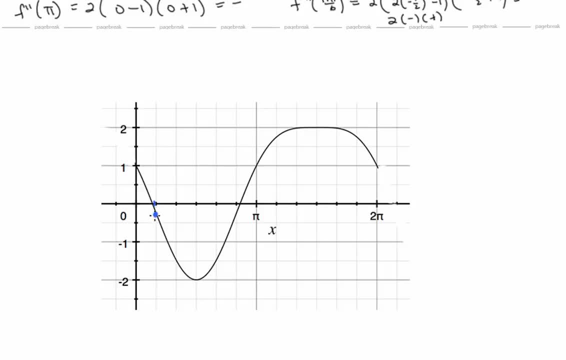 So here's pi over 6.. Here's our first inflection point. Here's 5 pi over 6.. Our other inflection point: we have concave down, concave up, concave down, And notice there's no change in concavity here at 3 pi over 2.. 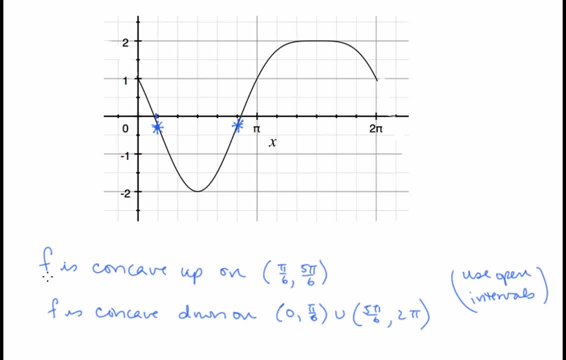 And so we'd say f is concave up on pi And notice there's no change in concavity here at 3, pi over 2.. So we're going to have an inflection point at pi over 6 to 5, pi over 6.. 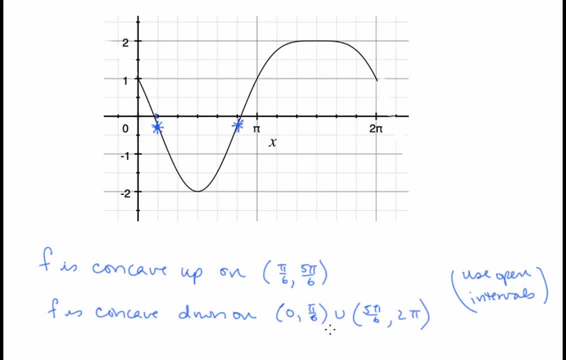 And f is concave down on 0 to pi over 6 union, 5 pi over 6 to 2 pi, And keep in mind that we use open intervals when talking about intervals of concavity, So we don't need to worry about the endpoints of 0 and 2 pi. 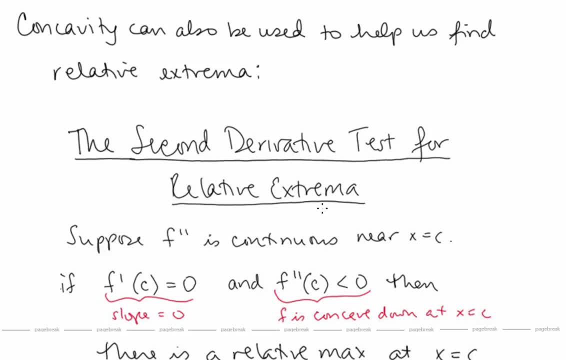 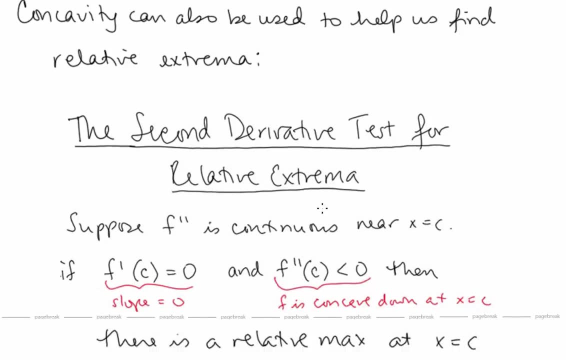 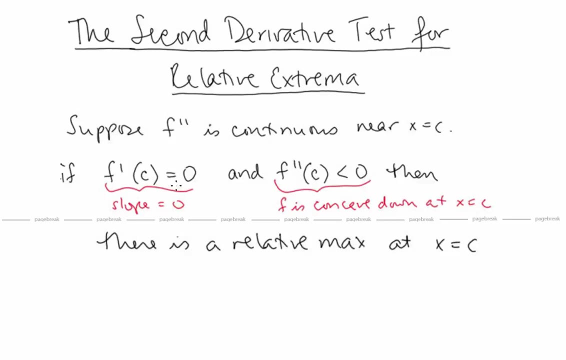 Now let's take a look at how concavity can give us information about relative extrema. Here we have the second derivative test for relative extrema. It says: suppose f double prime is continuous Near x equals c If f prime of c is equal to 0, meaning the slope of f is equal to 0.. 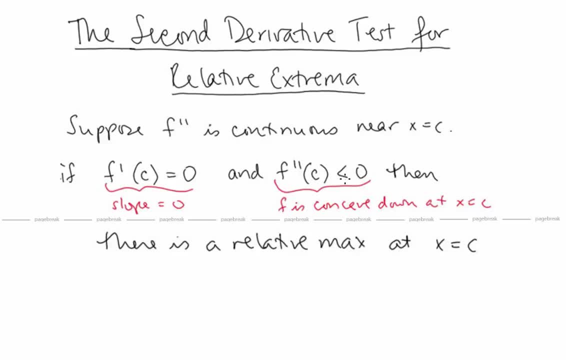 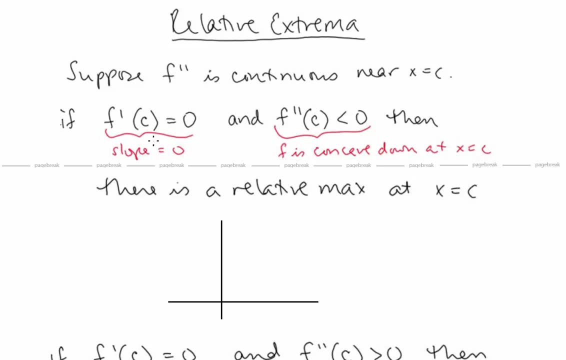 And f double prime of c is negative, meaning f is concave down at that point. Then there is a relative max at x equals c. So what we're saying is that the slope of f is equal to 0 at x equals c. 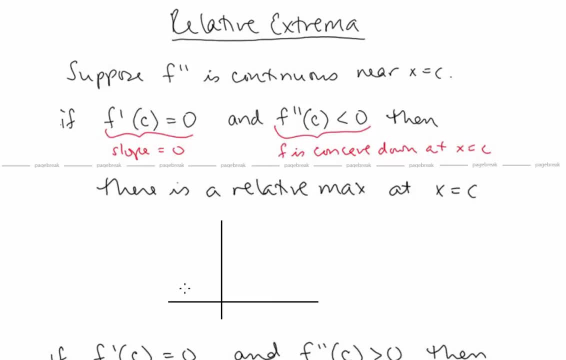 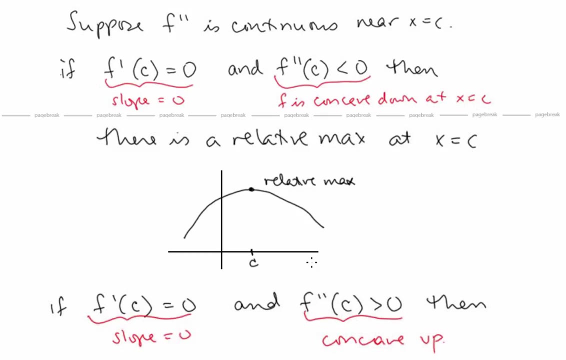 And f is concave down at that point. So it must be that we have this kind of situation And that we have a relative max. a relative max Slope is 0 and f is concave down. Similarly, if the slope is equal to, 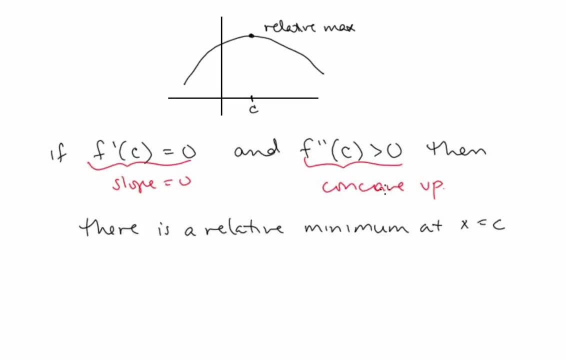 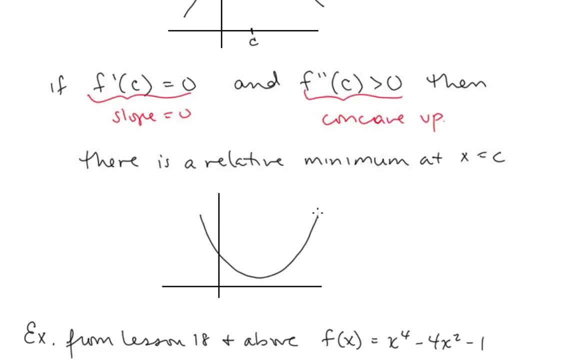 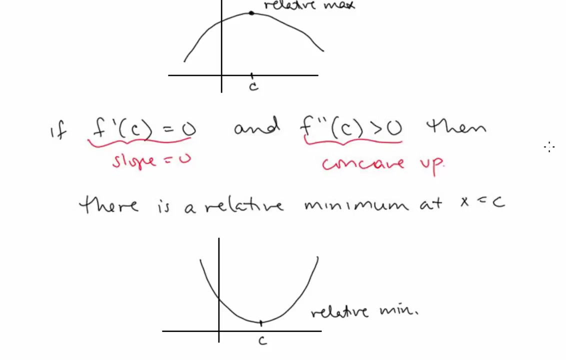 0 and f. double prime is positive, meaning f is concave up, there is a relative minimum at x equals c, So we have: slope is equal to 0 and f is concave up at x equals c, so we have a relative minimum. So this is what the second derivative test tells us, and it's 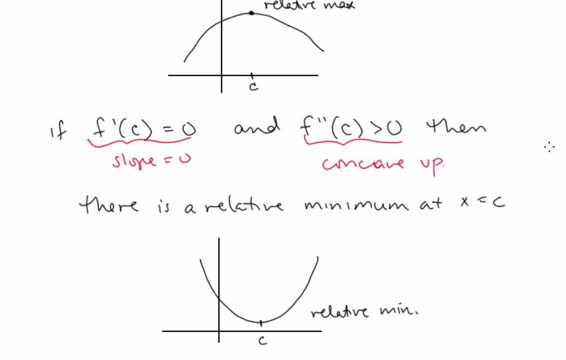 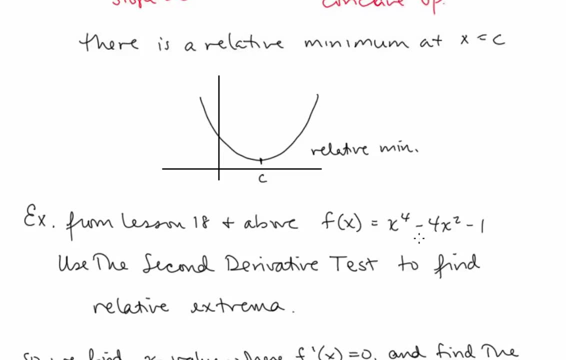 about relative extrema. It uses concavity to give us information about relative extrema. So now let's take another look at f of x equals x to the fourth minus 4x squared minus 1.. We looked at this problem earlier and talked about concavity, and we also saw it in lesson. 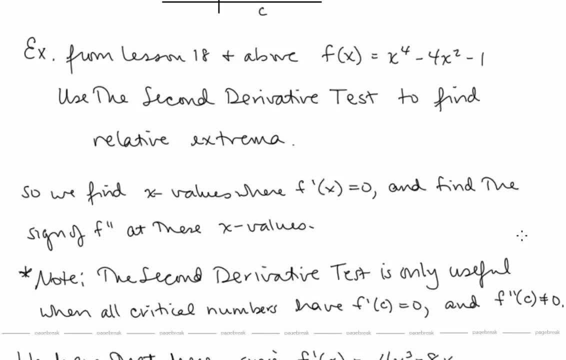 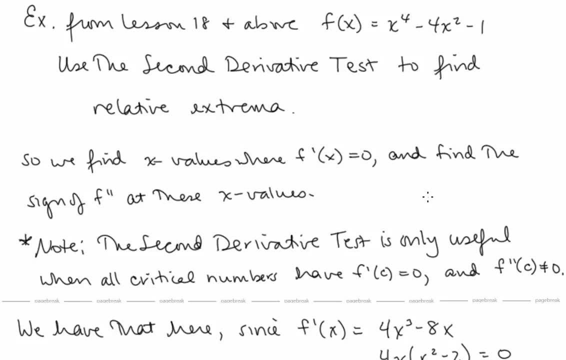 18 and talked about relative extrema. Now let's use the second derivative test to find any relative extrema. So what we need to do to use the second derivative test is to find any x values where the derivative is equal to 0.. 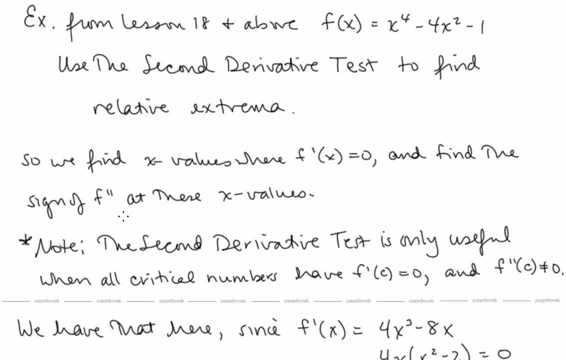 So we're going to find the derivative at x equals 0, and then find the sine of f double prime at these x values. So keep in mind that the second derivative test is only really useful when all the critical numbers have f prime equaling 0, and that the second derivative 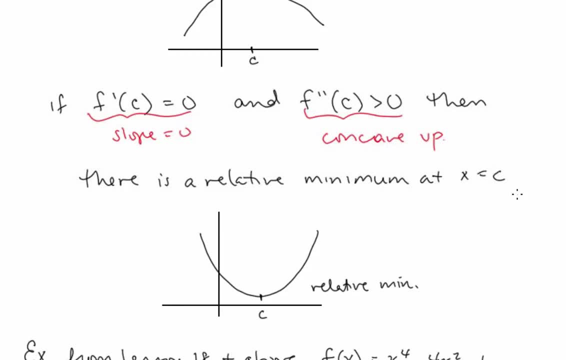 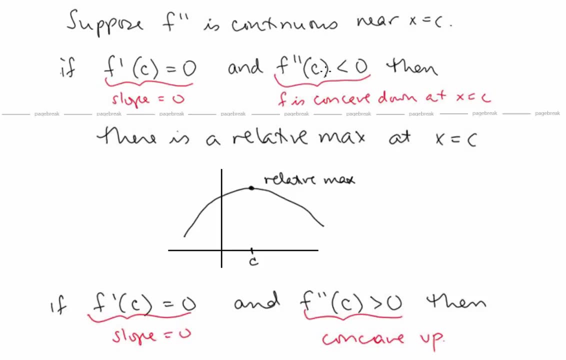 at those points is not 0. Because, remember, the second derivative test only gives us information for when f prime of c is equal to 0 and f double prime is either negative or positive. This is the only information we have for the second derivative test, so the only time it's. 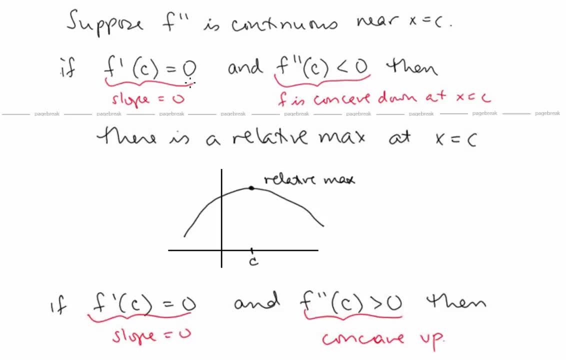 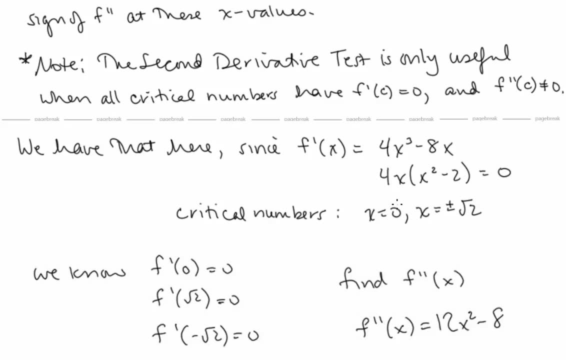 useful is when all our critical numbers come from f prime being 0 and f double prime at these points is not 0.. So we have that in this case, because we have our first derivative equal to 4x, to the third minus 8x, Factoring and solving for x, we have x equals 0 and x equals positive. and 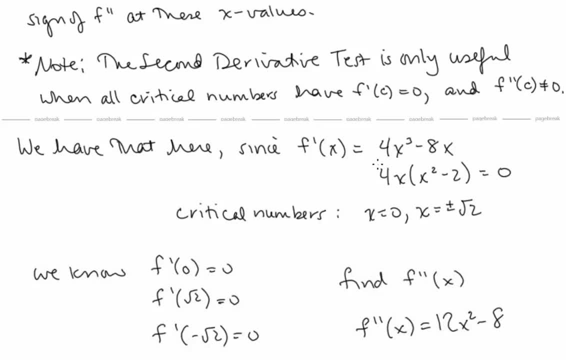 negative radical 2.. These are the only critical numbers, because f prime of x always exists And so we know that f prime is equal to 0 at these 3x values, and so we want to find and plug these x values into f double prime so we can see the sign. 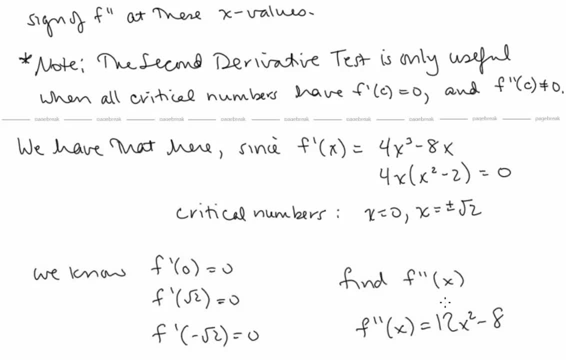 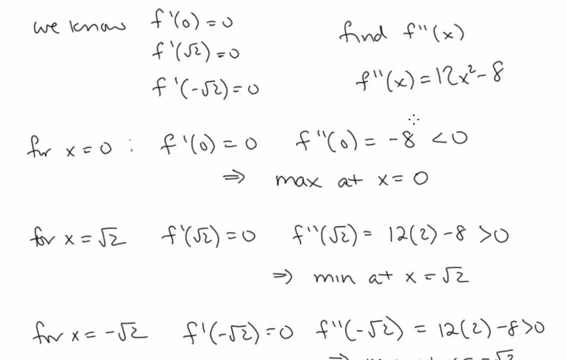 So f double prime is 12x squared minus 8.. And so at x equals 0,. we see that f double prime of 0 is equal to negative 8. And so that's negative and that tells us there's a maximum at x equals 0.. 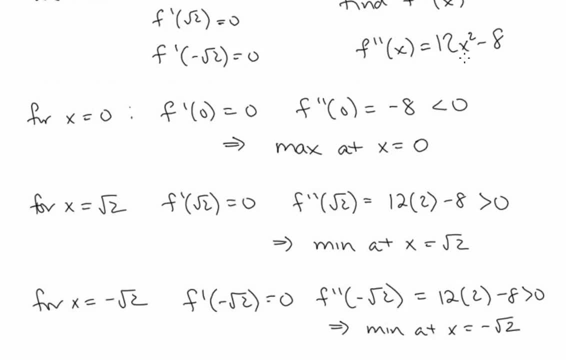 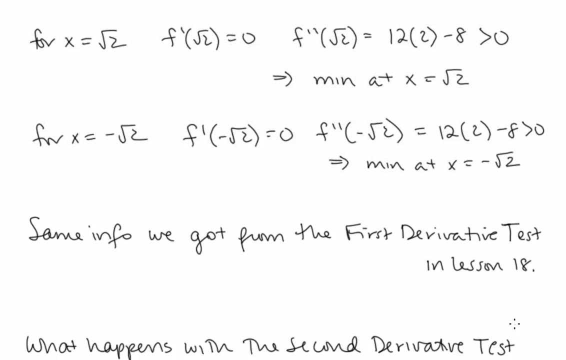 At positive and negative. radical 2, plugging into f double prime, gives us 12 times 2 minus 8.. And so that's positive, and we have minimums at these values, And so this is the same information we got from the first derivative test that we used in Lesson 18..